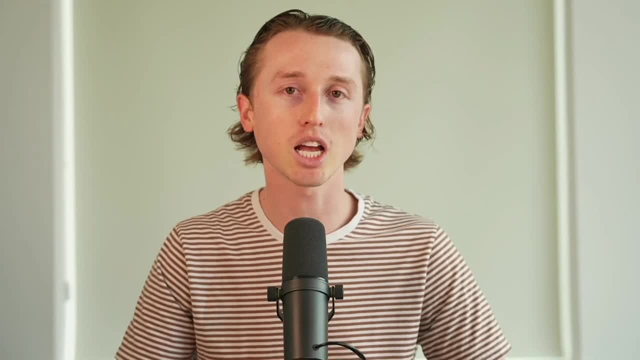 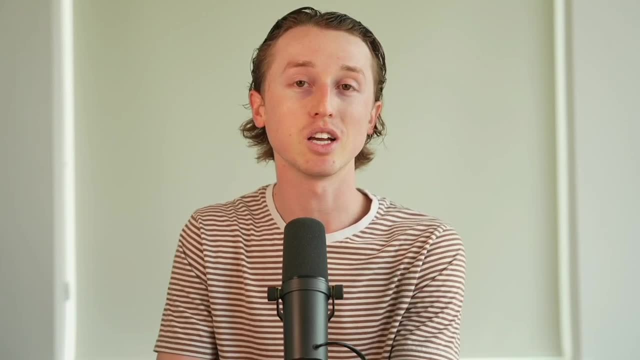 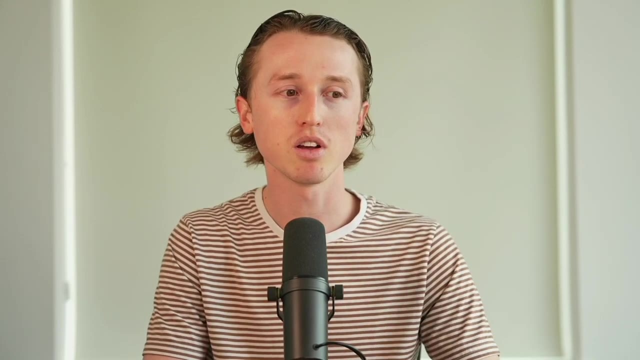 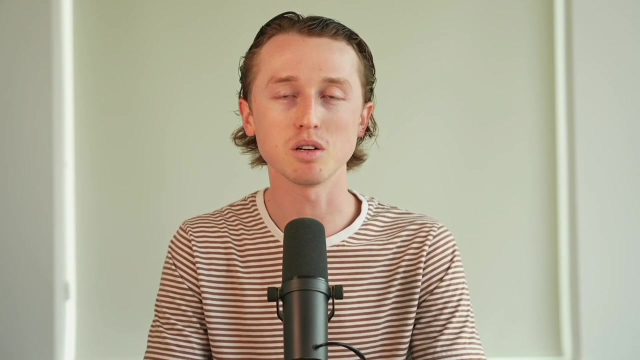 from the illusion of self and reach that God, state consciousness yoking oneself, which the word yoga means in Sanskrit to Brahman, the supreme deity, the God deity, and it's not the God deity of the Bible or Christianity, it's not the God deity of Islam and and Allah, it's not the God deity of of Buddha and Buddhism. 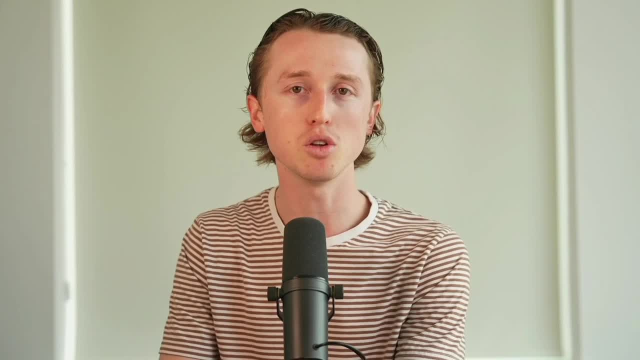 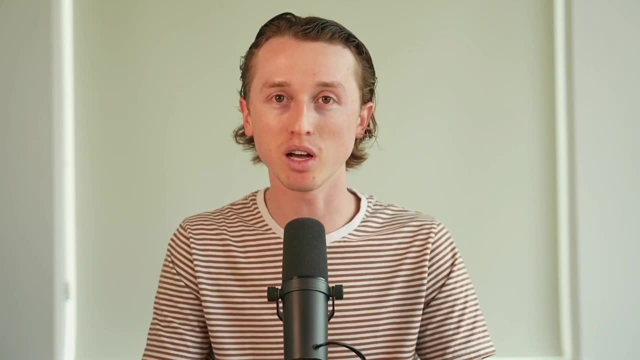 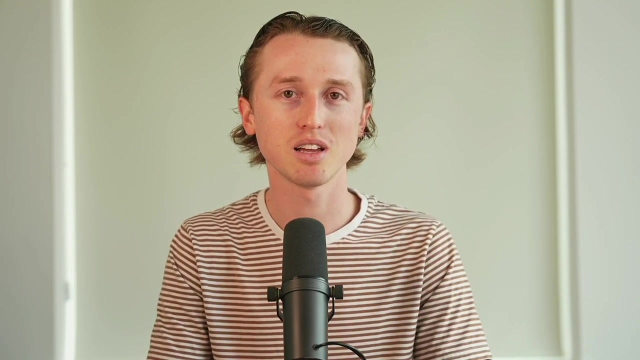 it's a specific deity, Brahman, in Hinduism, that you yoke yourself to by adopting the spiritual disciplines. the physical stretching part of yoga is actually just to prepare the yogi's body for to reach that deep meditative state more easily, to be more conducive to reach the state of moksha. 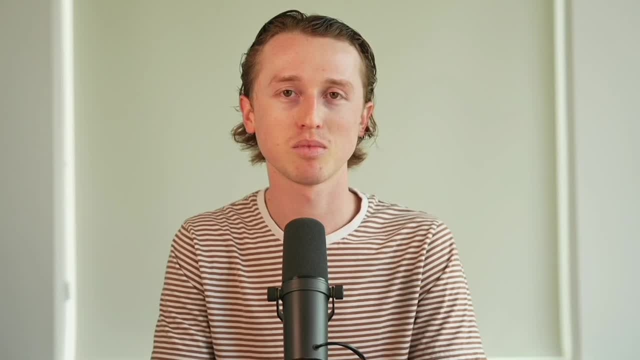 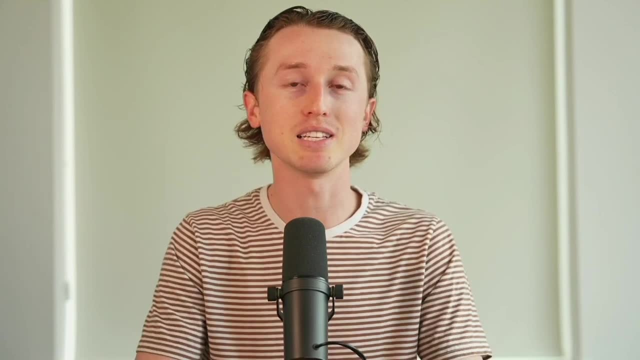 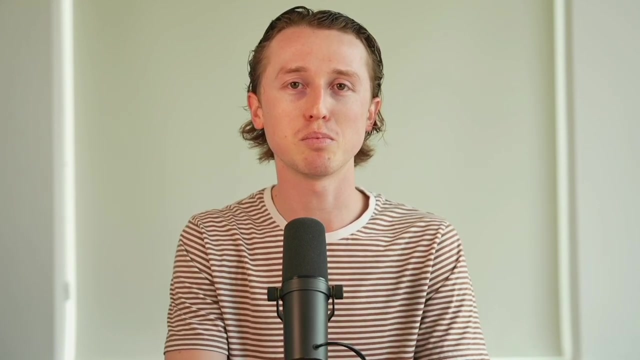 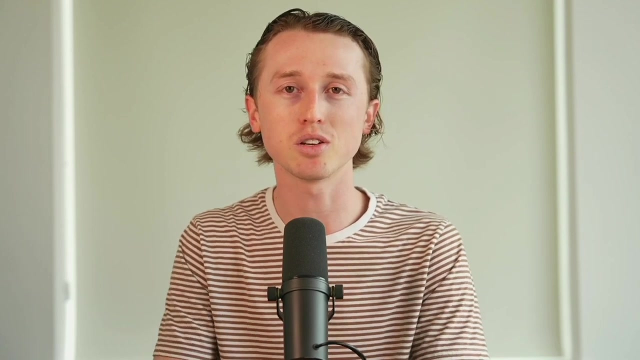 bliss union with Brahman. so they don't get to own, and they don't own spiritually in a legal, right sense of the enemy of Satan. they don't own specific basic human poses and then, as a result, it doesn't make it inherently demonic or spiritual spiritually dangerous, or you're opening a door when you engage in Hinduism and you believe and 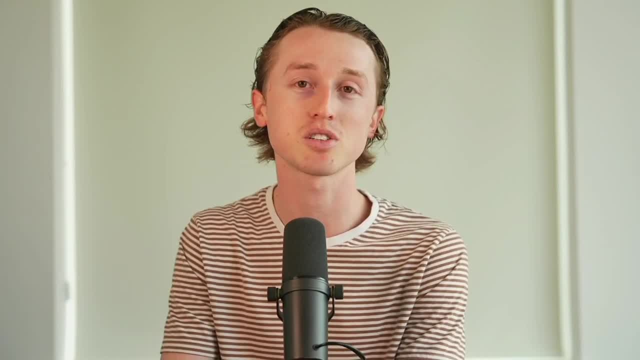 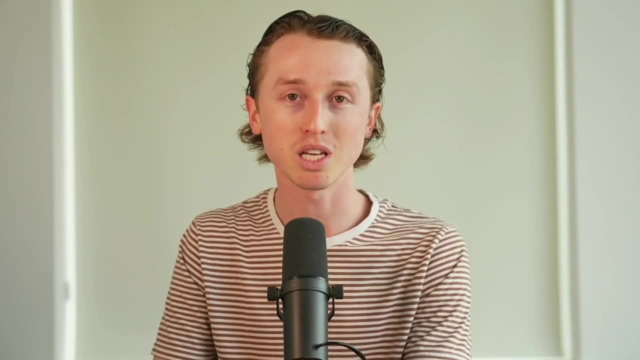 connect your faith to the spiritual discipline of Hinduism to free yourself from suffering through reaching moksha, the state of Bliss and enlightenment. by merging yourself, being yoked, to the God, consciousness, Brahman, then you're opening doors to these spirits. now I've seen these spirits cast. 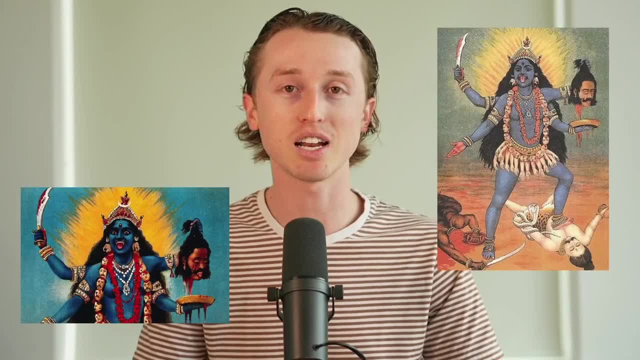 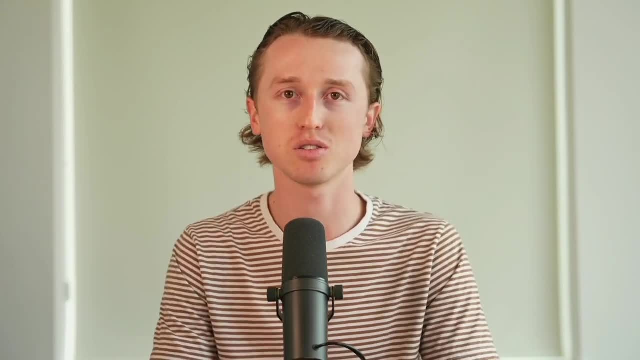 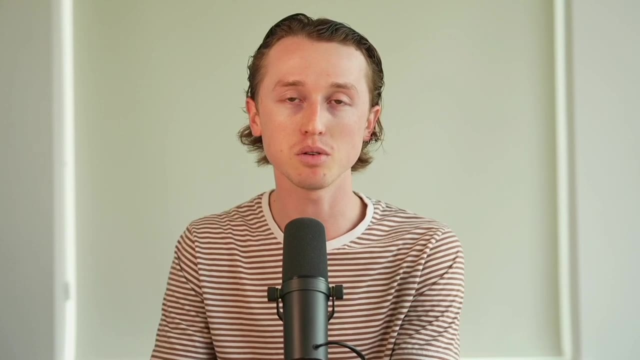 out of people. I've seen Kali the, the goddess that looks like that- literally get cast out of people and they're doing that. you know intelligent people who've been yoga instructors, who got really into yoga, and many, many times these spirits when you, when you truly engage in Hinduism and yoga and 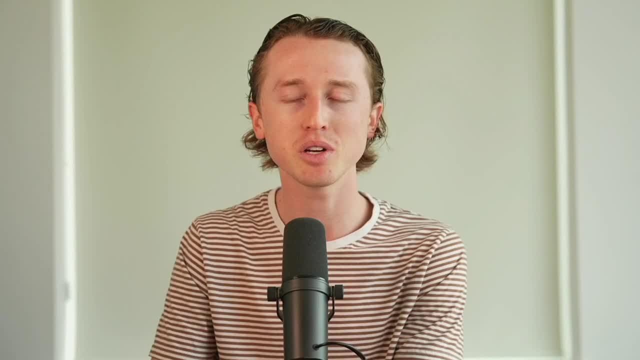 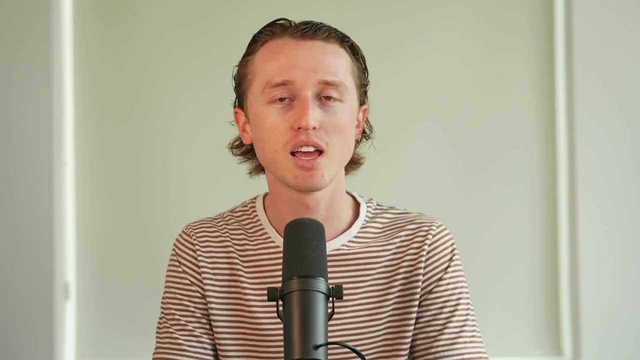 you're, you're, you're doing this practice. you're not fully attached to it, you're not fully believing some of these doctrines, but you're really getting into it. you're doing it just as they say. then you begin to actually open doors and these spirits will fill you and they'll begin to kind of force. 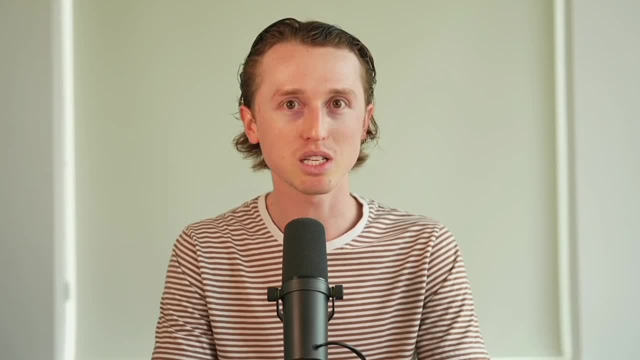 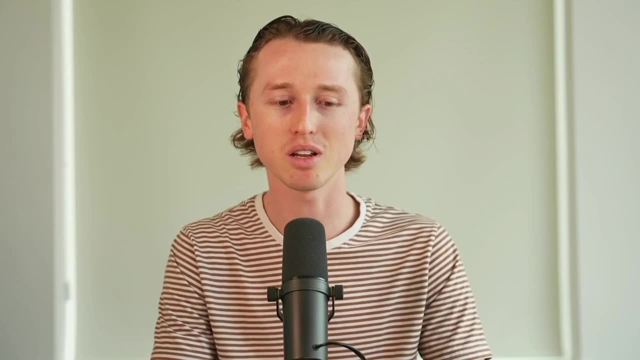 yoga, where, if you don't do it, your body starts to ache, you get really tense, your body starts to not feel good. yet there's people who never do yoga and they, they're great, they're limber, they're healthy. now that's. you can't generalize, because there's some people who don't even eat great yet. 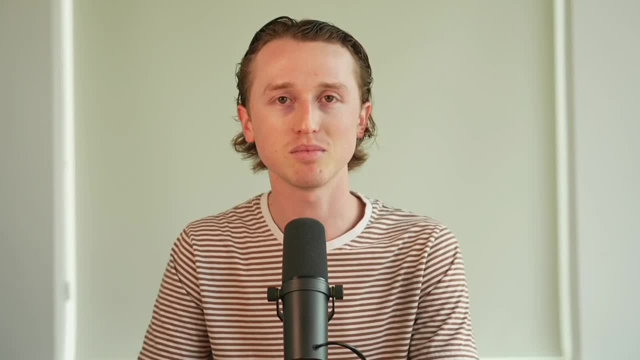 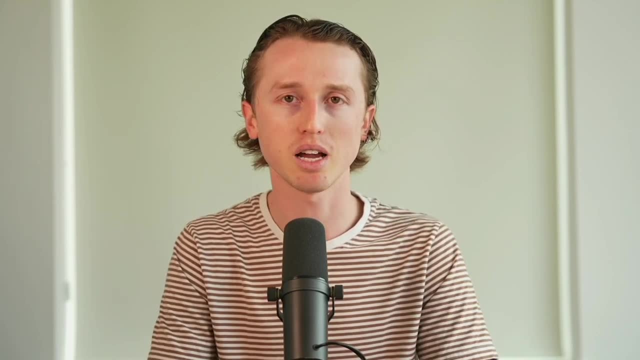 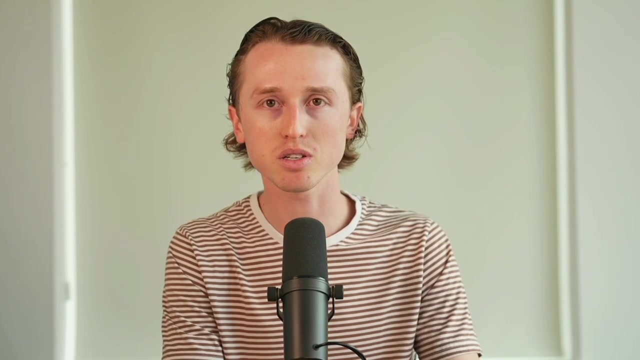 they feel great and they live long. then there's people who do that and they develop disease very quickly. so it's always better to be healthy as a as a just, as a baseline. but when you get deep into the spirituality of yoga, not just the physical poses, you can go to physical therapy and do the physical poses to help you know. 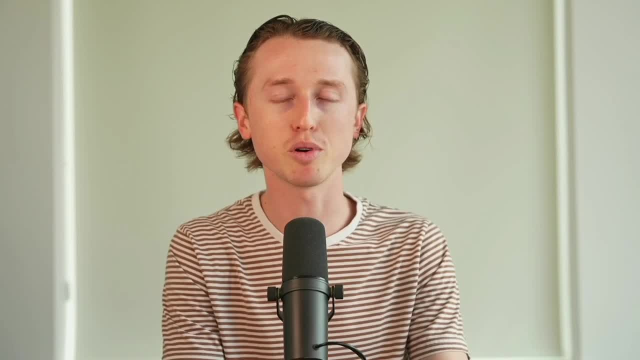 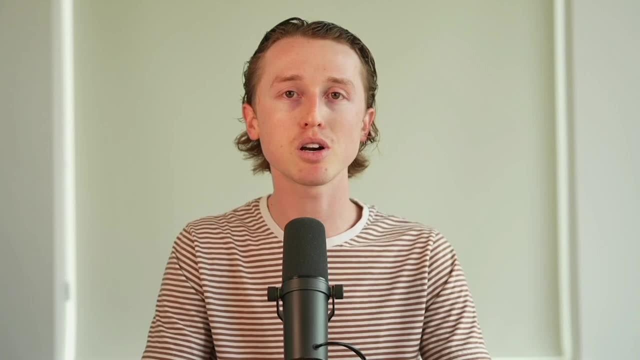 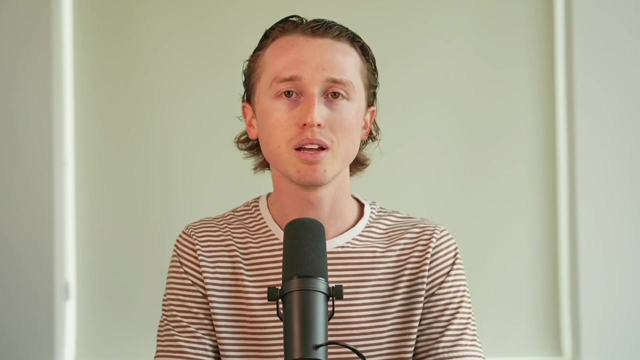 whatever condition you might be facing, in a very non-spiritual way, a very just anatomical way, and in modern yoga, as it's come to the west, it's merged with Anatomy, it's merged with kinesiology, it's merged with different, you know, practices and medicinal practices, physical therapy, and there's 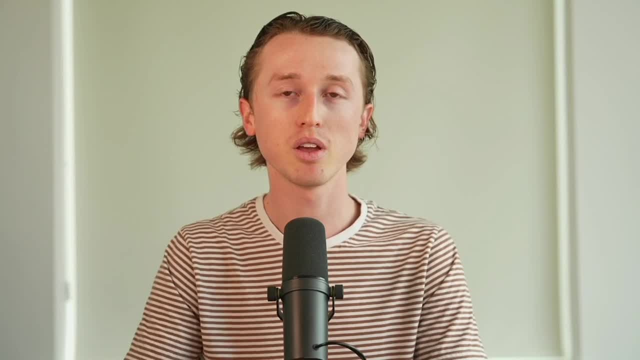 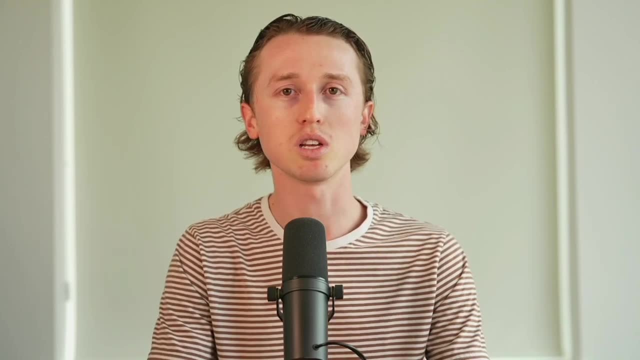 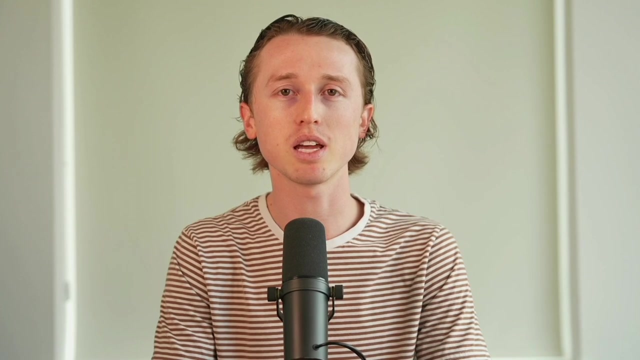 been more research on some of the poses that yoga decides to do and seen some of the benefits that the anatomy on on specific parts of the body. you know: loosening the, the fascia throughout the body, the ligaments and and different muscle groups and all these different things. so there is actually- and 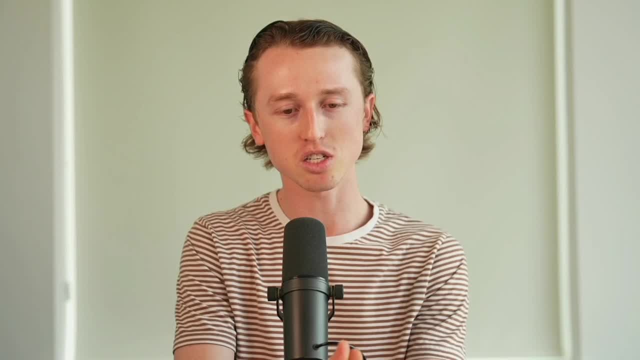 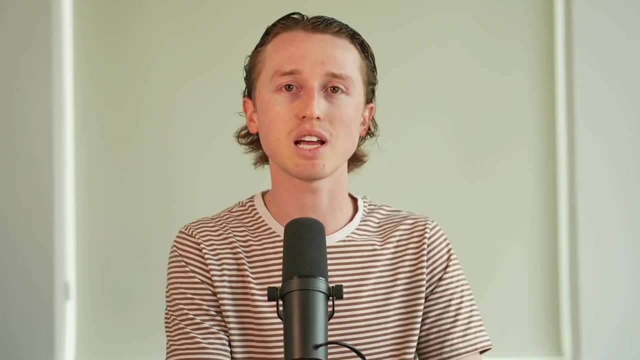 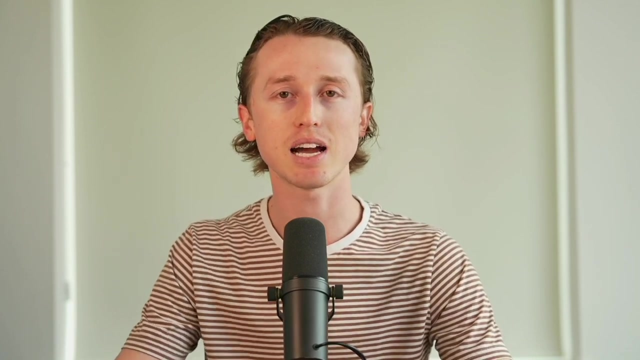 the small tweaks to your heel and where you put your toe in relation to your heel and stacking the knee over the over the foot causes this to be activated. there's a lot of physical, actual, scientific understanding about the Anatomy of certain poses that Hinduism and yoga decides to use, but just because they decide to use it doesn't mean it's now off limits. 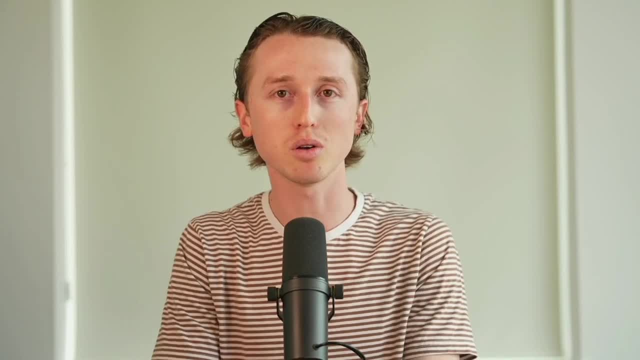 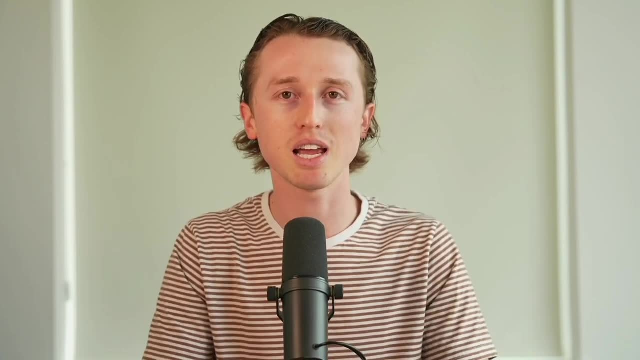 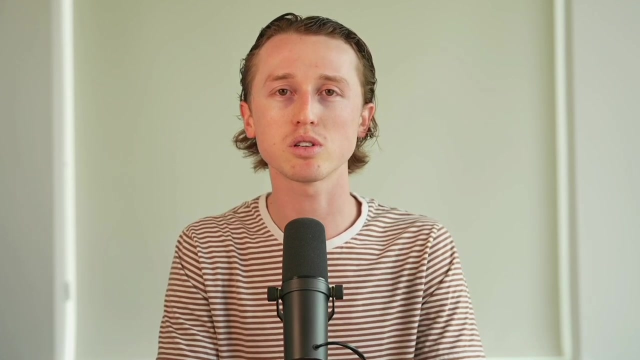 or inherently owned by them. it can be used for the glory of God. all things do for the glory of God. it can be used to benefit your health, to stay limber, to stay healthy, to stay flexible. so stretching your hamstrings, stretching your lower back, stretching your shoulders and your neck, and and staying. 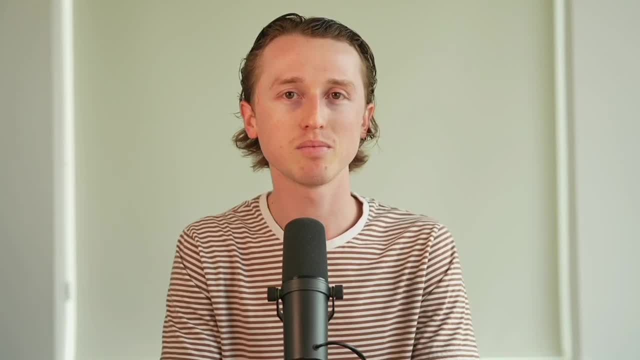 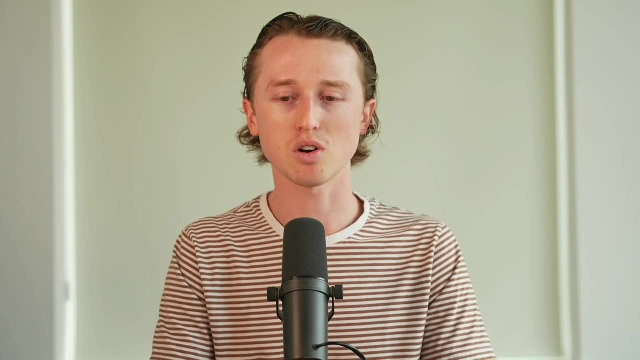 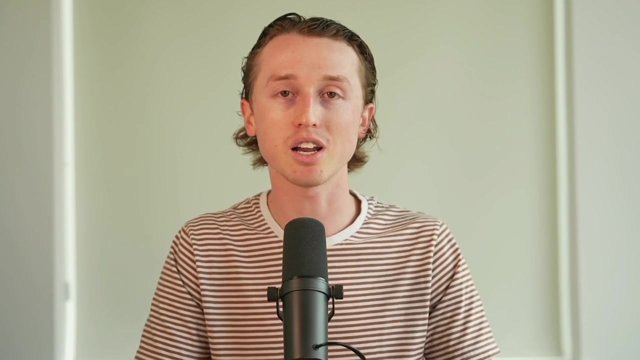 healthy and limber is not practicing yoga. you're not merging yourself to the God Consciousness. you're not yoking yourself to Brahman. you're not trying to realize that this life is an illusion and that the key to suffering is to realize that you are actually God and the self is an illusion. you're not believing that you're doing. 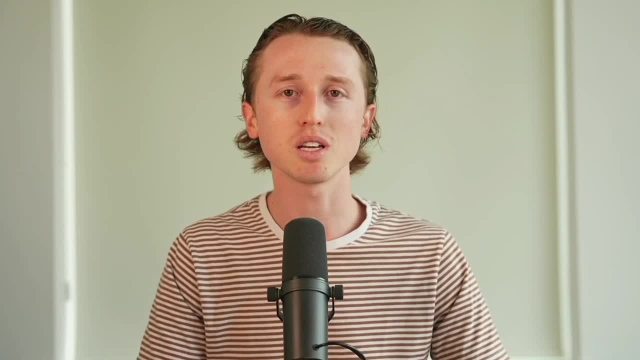 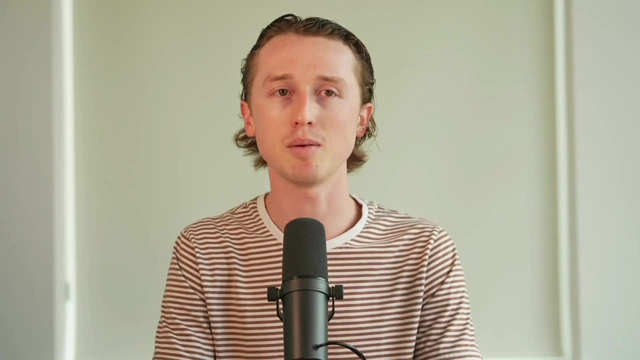 it because you want to be healthy. you're doing it because you want to have longevity. you're doing it because you want to live long and you want to keep the Temple of the Holy Spirit, your body, in good health, because you're sitting all the time or you've gone through. 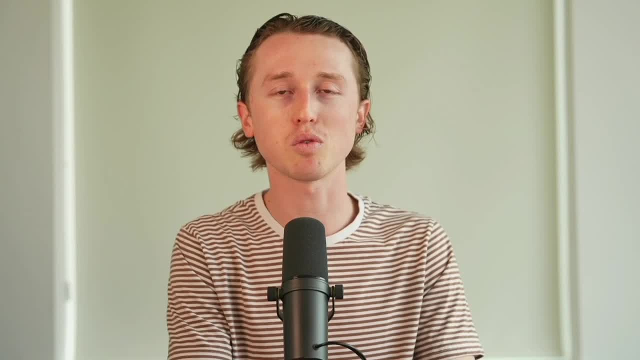 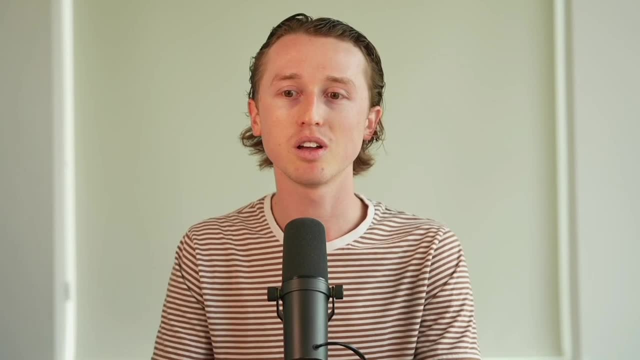 physical injury and you want you're doing a specific stretch for that reason doesn't mean you're practicing yoga. but the problem is a lot of people call regular stretching now yoga because they don't use it and the word properly how it's actually used in Hinduism, how it's been used for 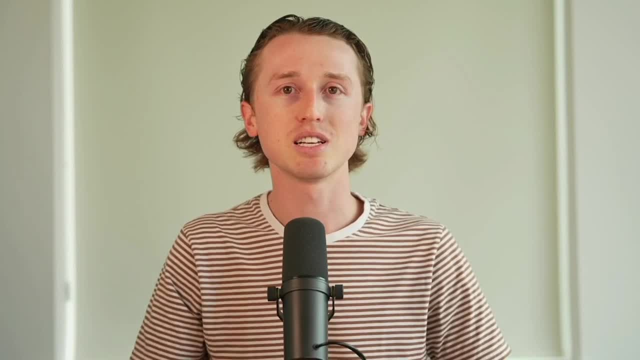 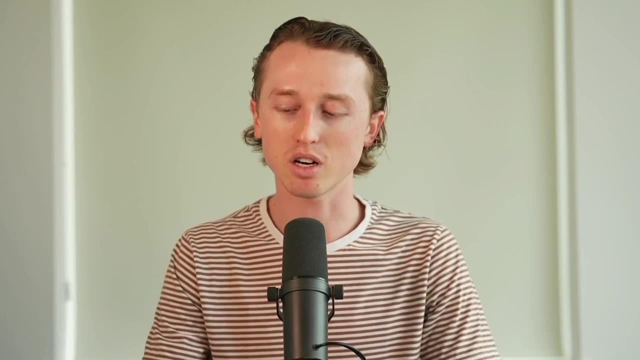 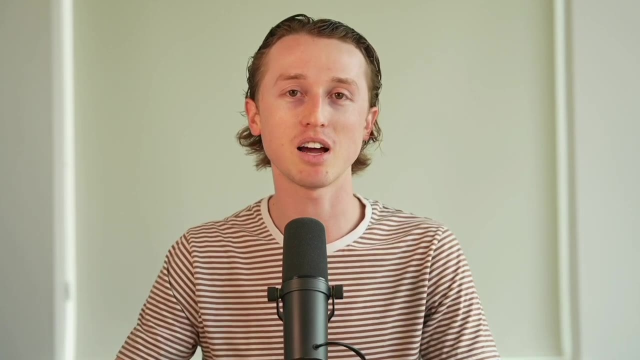 thousands of years since it came to the West, this kind of secular version of yoga actually, where I remember when I was becoming a certified yoga instructor, the- the studio that I was doing was a studio that I was doing it at- had like this very distasteful view of this new studio that came in. 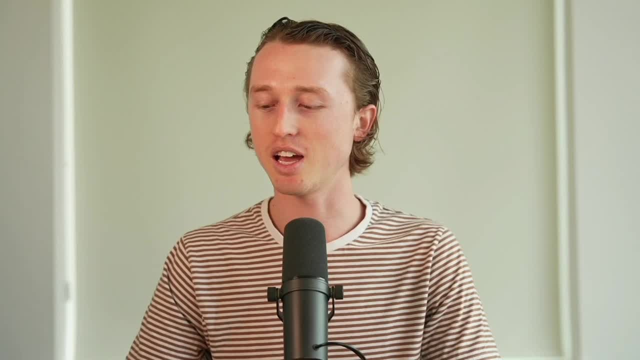 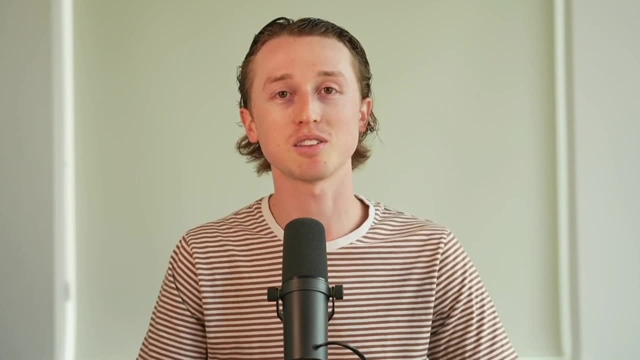 town and it was called like bulldog yoga or something and the distasteful view was there because bulldog yoga was like we do yoga, but with no spiritual. that was like their slogan: they're not the spiritual side, just for the stretching and we were like man. that's lame. 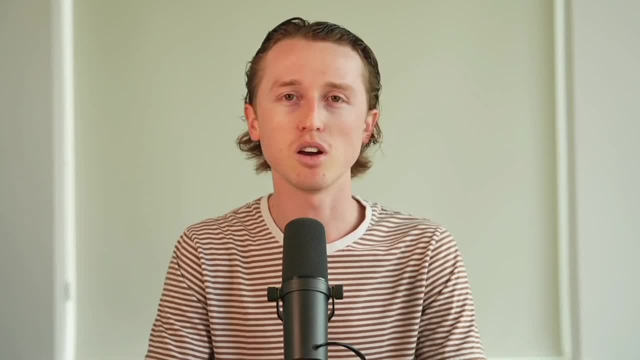 like they're totally just spitting in the face of the ancient, you know Hindu practice and like man, that's just. there was a distasteful view of it, like that's not cool, that's kind of disrespecting the, the sanctity of of Hinduism. 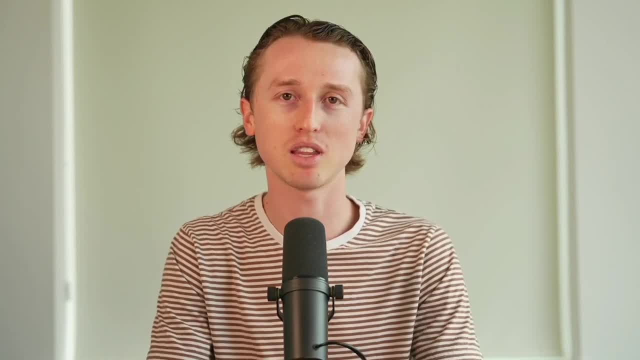 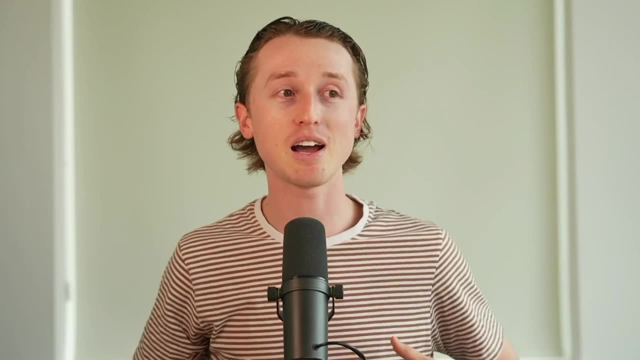 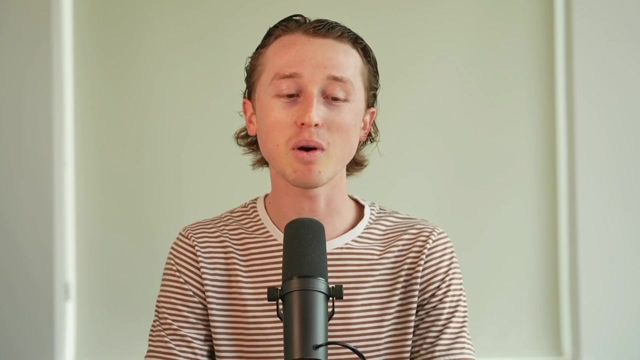 and true yoga. it's not true yoga, like you can't call it that. so they're even that view amongst the true yogis. for those who are kind of trying to make it all just physical and non-spiritual and now understanding more of the kind of the spiritual realm and the spiritual things, I'm 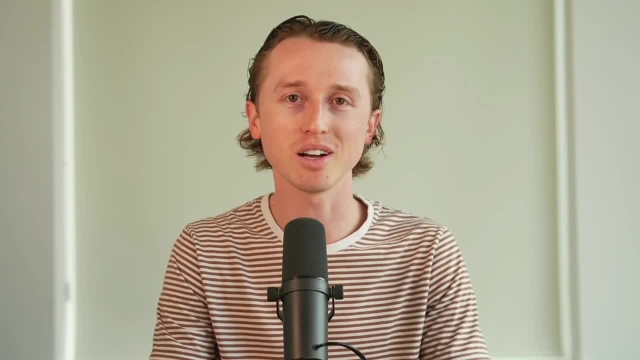 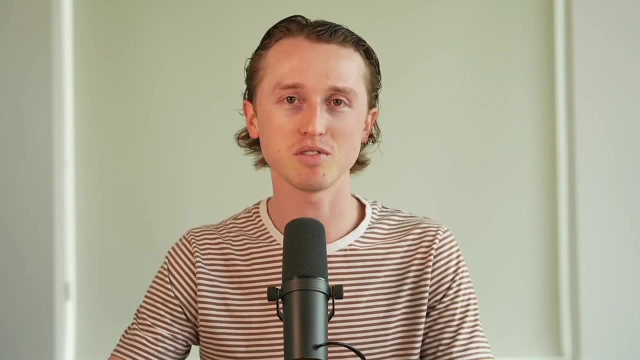 like wow, that kind of they were going in a better direction. but just drop the word yoga, because it's a great word for being yoked to and it's connected for the long lineage of thousands of years going back to the Upanishads and the Vedic scriptures and the ancient yogis of Hinduism. so you don't. 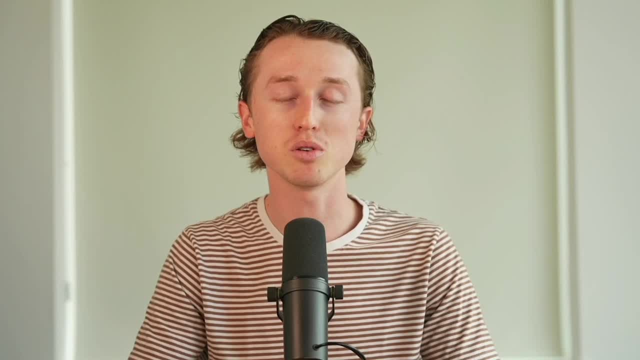 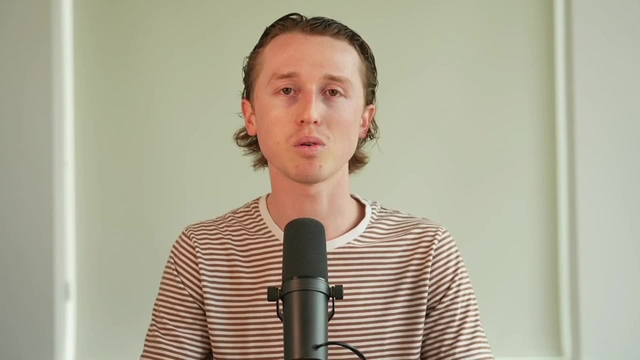 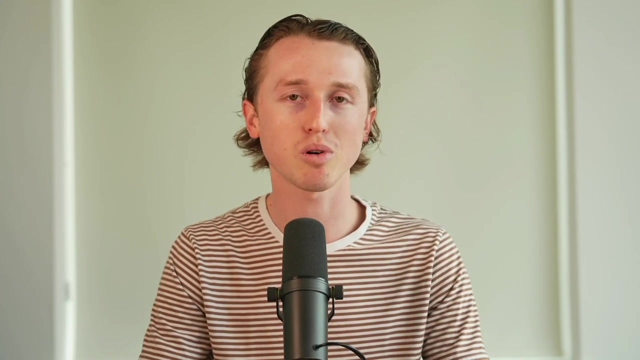 have to use that term now I believe there will be a new term that people use, because a lot of the stretches and physical postures that are done are beneficial for somebody's health and their longevity and staying limber. that's why people stretch after workouts. that's why, if you play 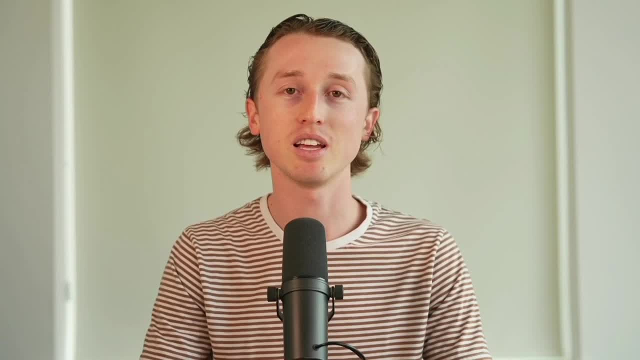 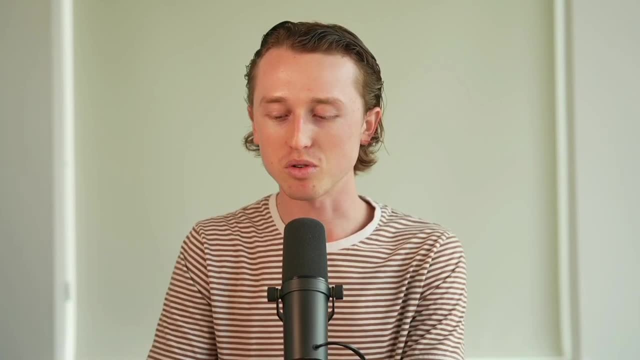 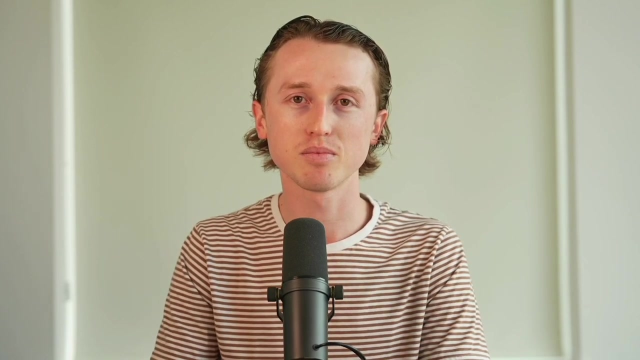 sports there's a lot of stretching involved, injury prevention- it's honestly really, really great. but when you get into the spiritual things, when you truly try to find your heart's pleasure in, in relaxing your mind, to reach this state of moksha, in adopting some of these ideas about Karma, maybe 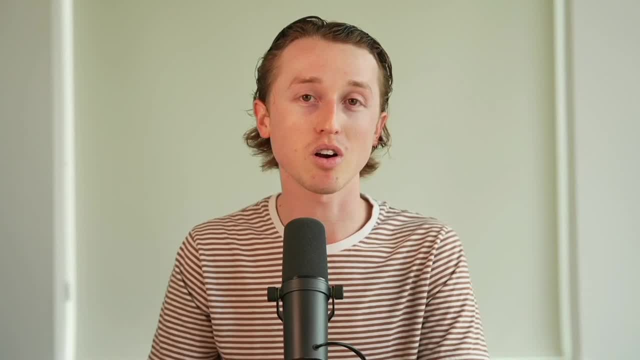 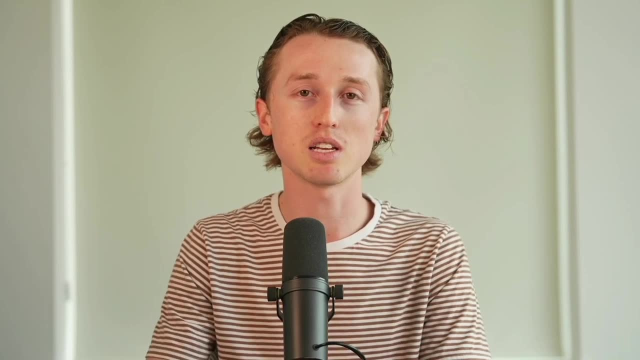 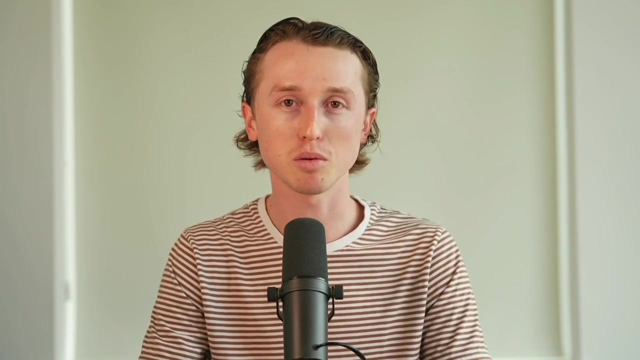 reincarnation, uh, cleansing yourself of karmic cycles and things that are stuck in you that need to be purged before reach the next level in the stages of reincarnation and you begin to really adopt the core doctrines that yoga is based upon. because, as I said, the physical aspect of stretching is merely to prepare. 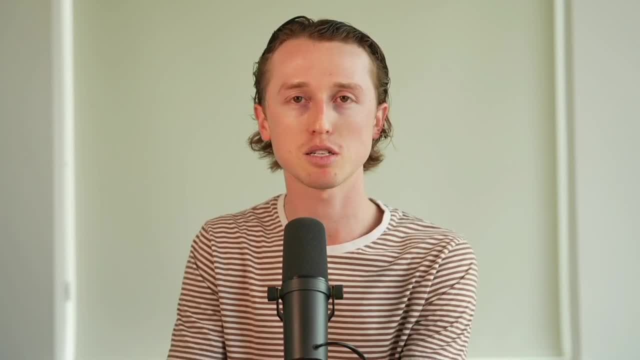 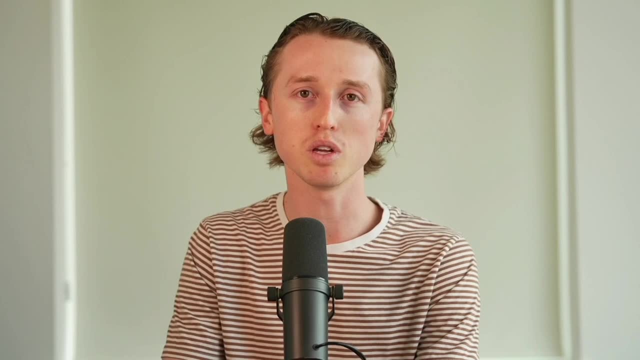 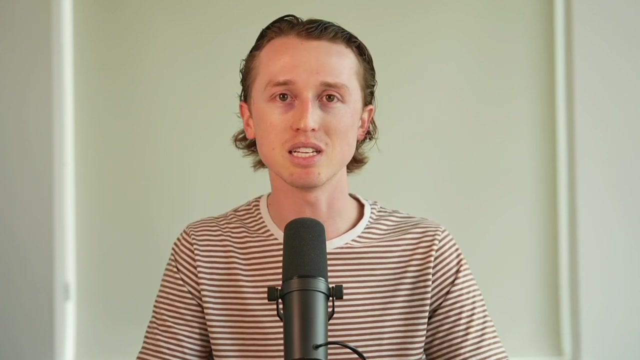 the yogi for that actual spiritual aspect, for that actual time of meditation where they try to reach the state of merging and union with brahman, the god deity- but then you've got bhakti- is just obviously inherently summoning deities. you're worshiping hindu deities, but there's no. 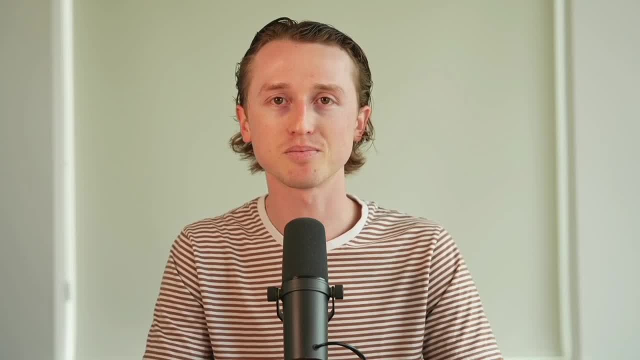 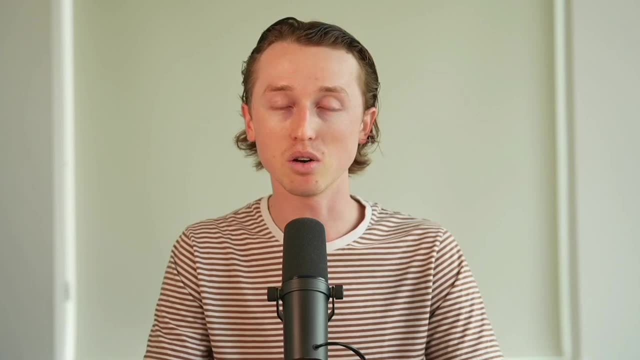 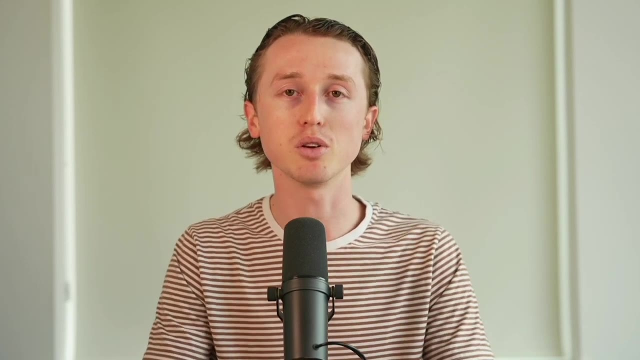 stretching involved in that. it's chanting, so, but that's bhakti yoga. then you've got ashtanga yoga and then you've got kundalini yoga, which is allowing a serpent to go up your spine and activate your, your third eye, your crown chakra, to bring you enlightenment. and people have kundalini. 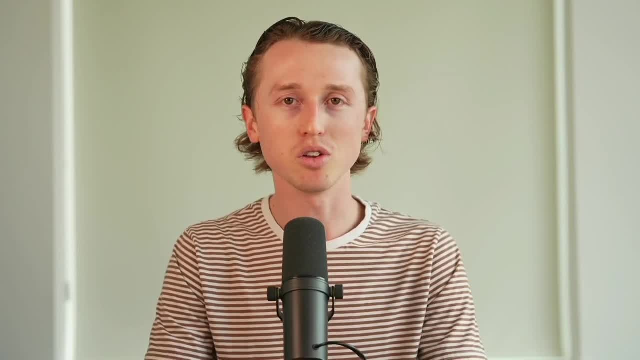 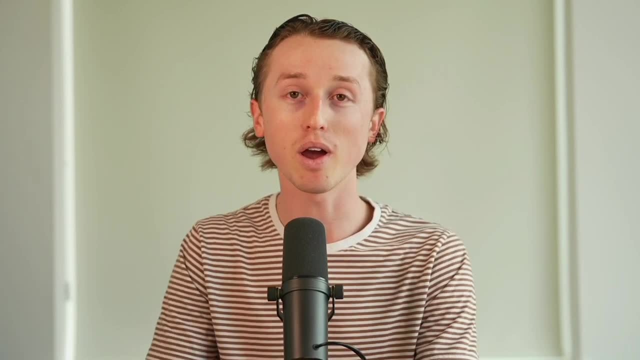 experiences, oneness, experiences which are, which are you don't want to get involved in, that the spirits will actually gain control of your spine. people have horrible pain afterwards when they try and get away from this, when they realize that, hey, this was not what i thought it was. this is- i'm not trying to open myself up to these thousands year old demons of of hinduism, and kundalini yoga is actually fairly recently formed, but it's still a version, an offshoot, of basic hinduism, which is a whole gamut of deities that are worshipped and people. 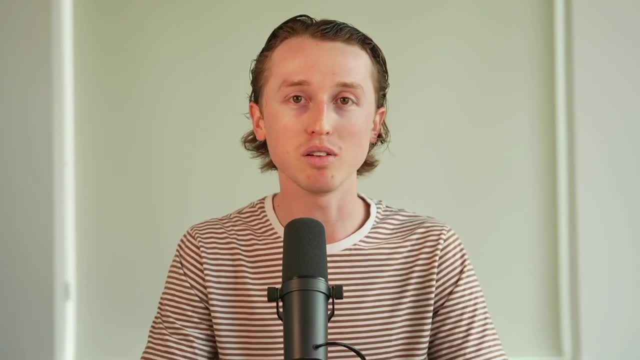 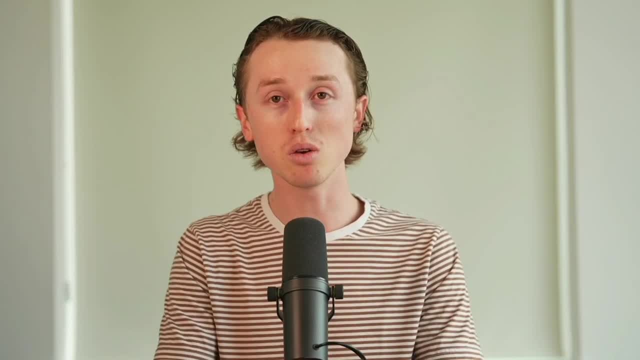 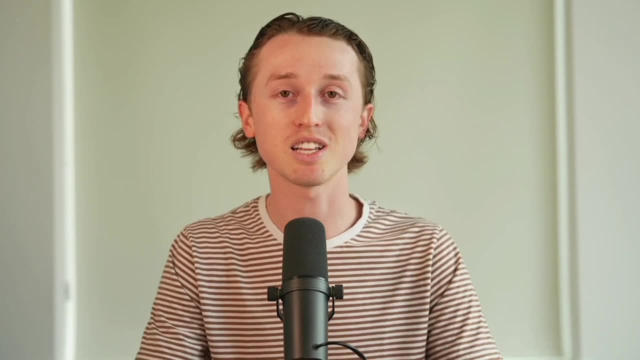 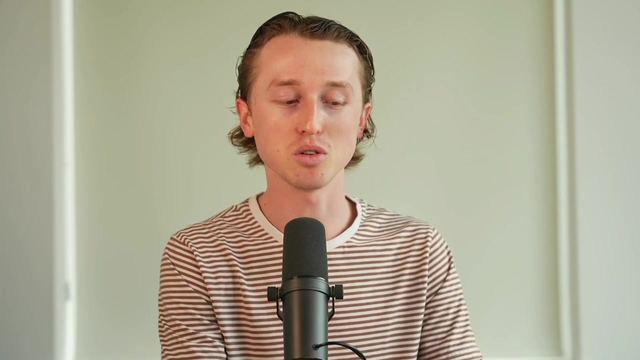 get to own basic human stretches. they merely use those for their desires. the same thing goes for you. you can use a basic human stretch that is anatomically, scientifically, beneficial for your body and injury prevention. for the glory of god, to keep the temple of the holy spirit healthy. 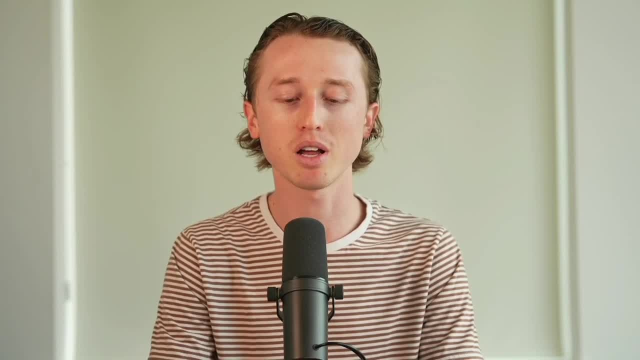 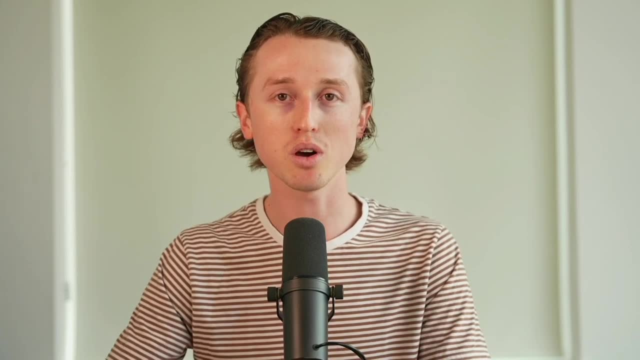 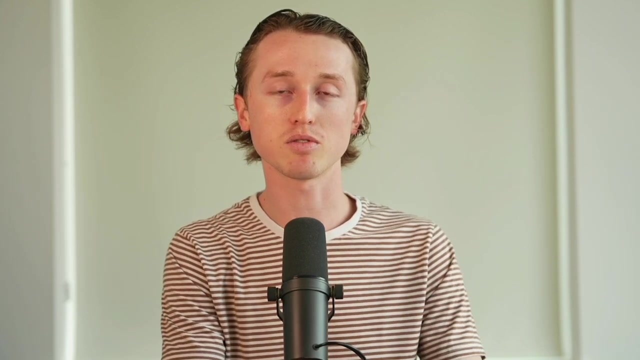 limber intact. it's not inherently demonic just because it's becoming popular now, because hinduism is becoming more popular in the west and that this word yoga is now like, seemingly attached to it. no, just get rid of the word yoga. study these things for their physical benefits, for their- you know- effects. 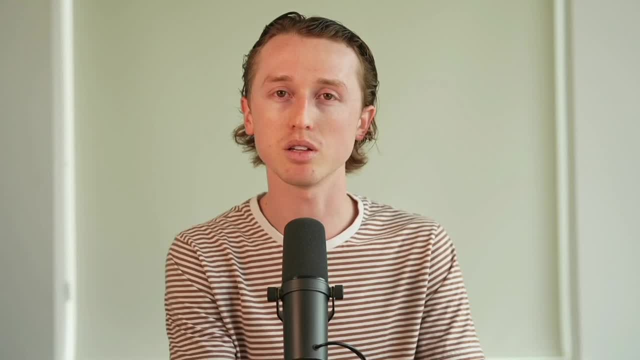 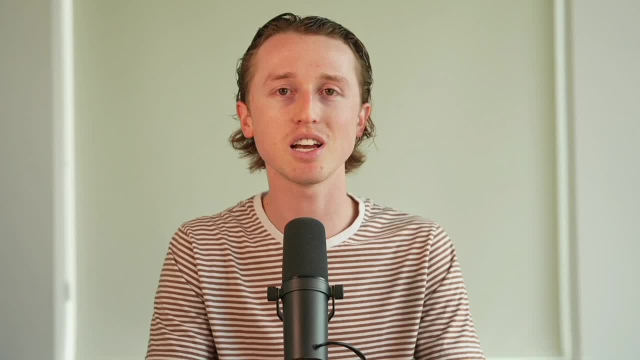 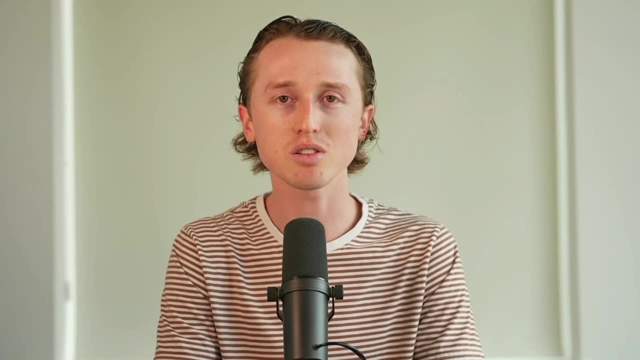 and just study it anatomically, like you're studying kinesiology and anatomy. you're, you're people. this is, this is physical therapy. physical therapists go to school for years to learn this stuff, to better the lives of people who are in pain, people who have chronic conditions. 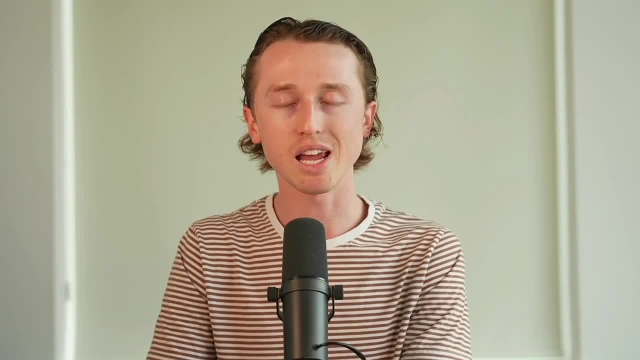 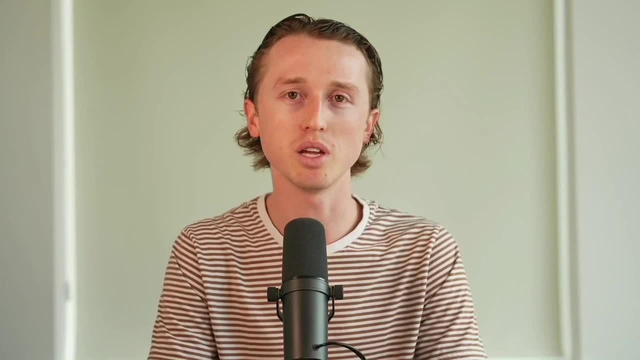 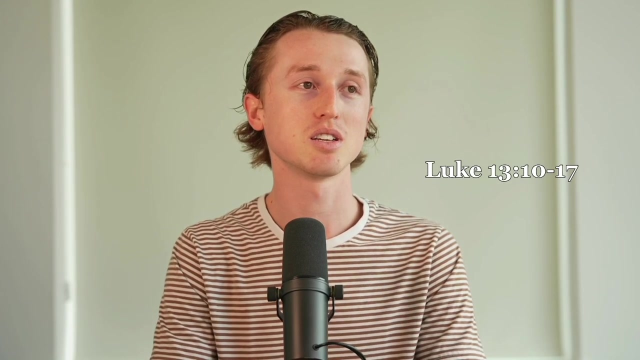 and never try and find the, the, the answer to healing in yoga or hinduism or this practice. always keep your eyes fixed on jesus, who is the true healer, like even a woman who, in the bible, we might have thought today, man, that that that girl needs yoga, that girl needs stretching that girl. 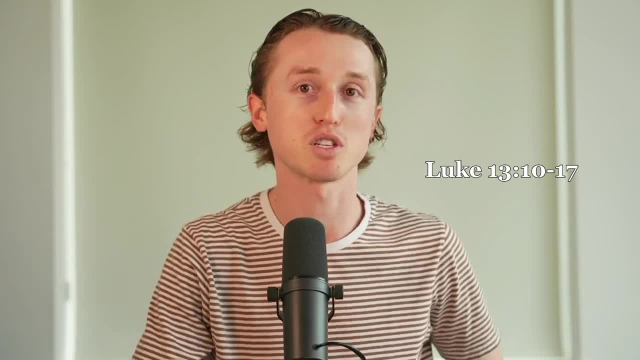 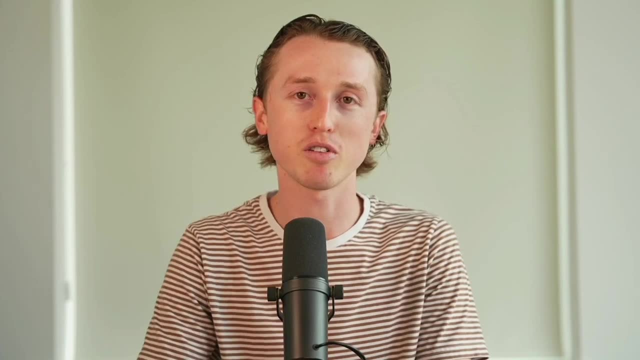 needs to, you know, open up her chest because she was bent over. but it was a spirit of infirmity that was causing that bend over where she couldn't, you know, and boom, jesus cast that spirit of infirmity out and she was great, she was fully healed from that day on. so jesus is the healer, this the 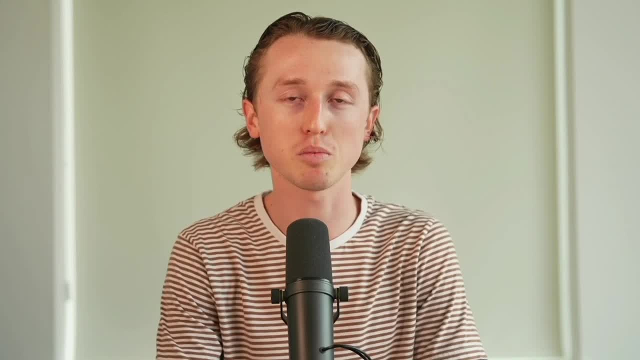 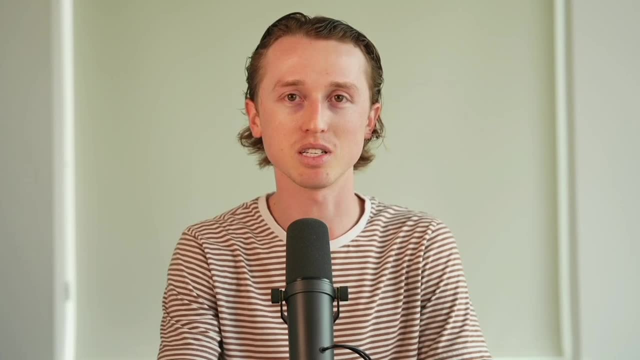 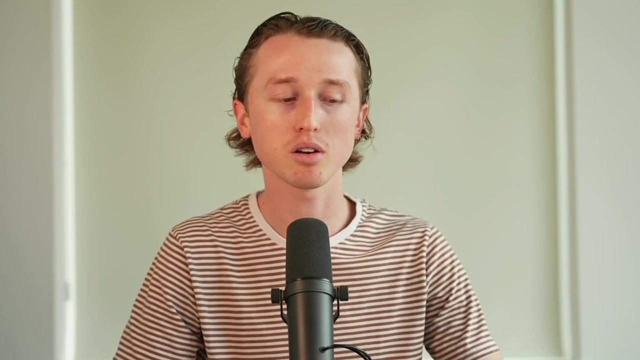 supernatural power of god, the supernatural power of the holy spirit to heal is real and that that should be our core aim. that should be our core fixed. uh gaze, because divine health comes from god, comes from jesus. by his stripes we are healed, but we can do things like eating better, use wisdom, but don't be so scared that you're opening up a 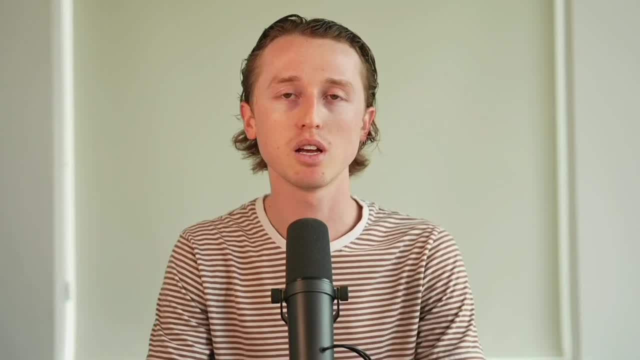 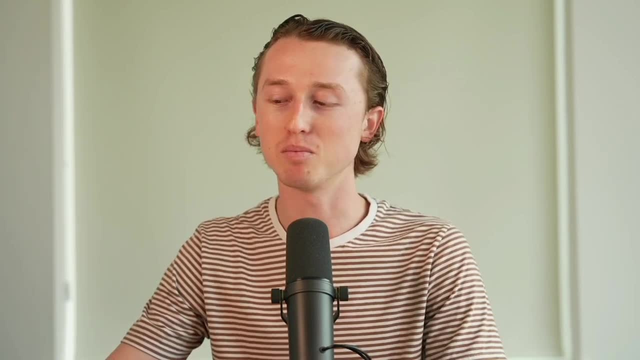 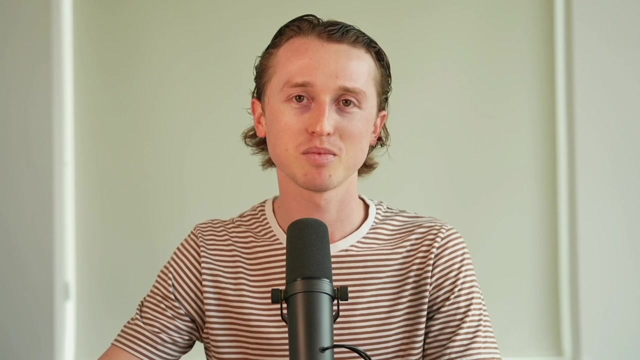 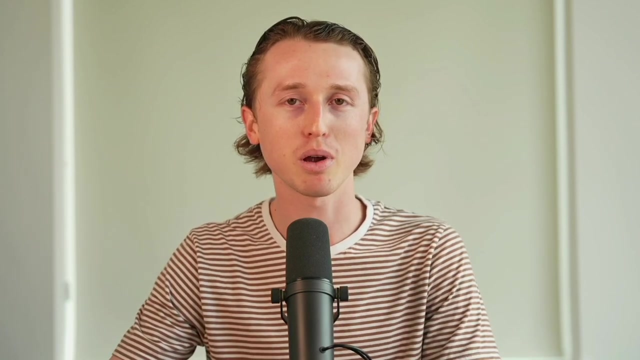 legal right to these demons, open doors to these beings just because you're doing a basic common stretch that happens to be done by hinduism, by yoga. they don't get to lay claim on every single basic human stretch. so, as a result, you can be healthy, you can stretch without having to be worried and paranoid that 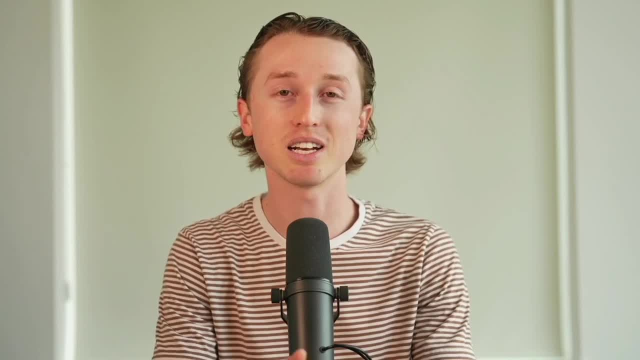 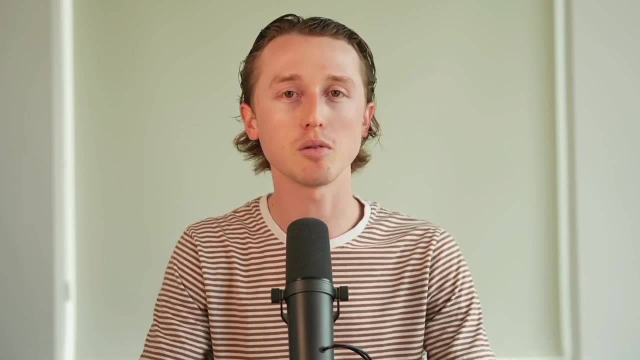 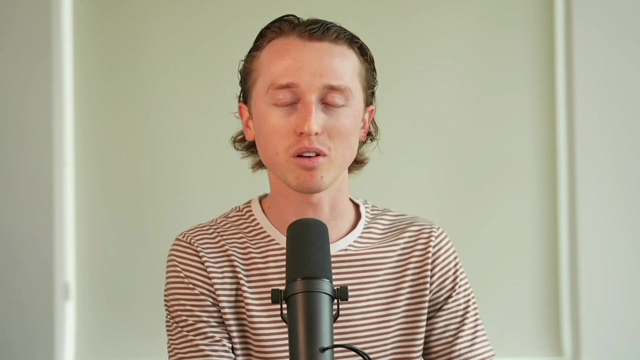 you're opening up doors to demons. if you're intentionally believing and attaching your faith to the doctrines of hinduism and yoga, then you're beginning to open up spiritual doors, then you're beginning to connect with other spirits that guide you in a different direction than the holy spirit. but do all things for the glory of god and like paul said when it came to 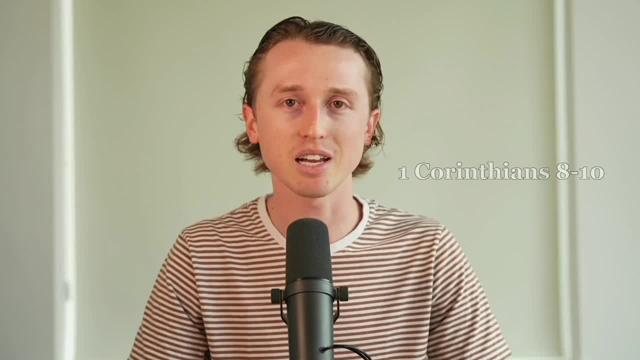 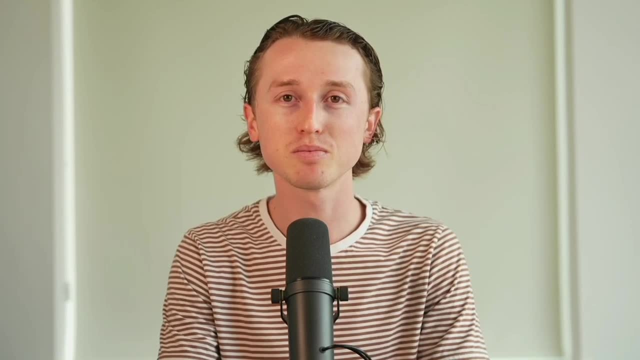 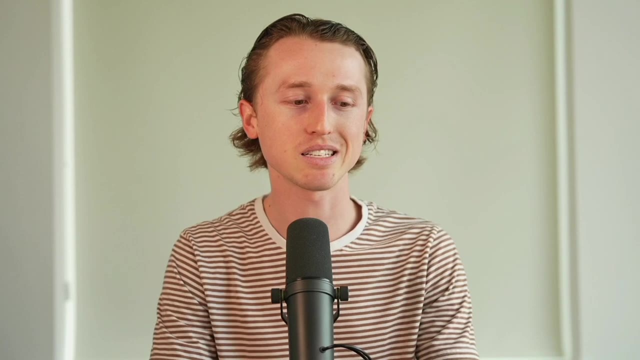 sacrificed. you know, food that was sacrificed to idols. he says: there's liberty in christ. there's liberty in christ. it may not, you know, be beneficial, but it's permissible. now, when it comes to stretching, just make sure that you're doing it for the glory of god, that it's not becoming an idol. you're becoming obsessed. 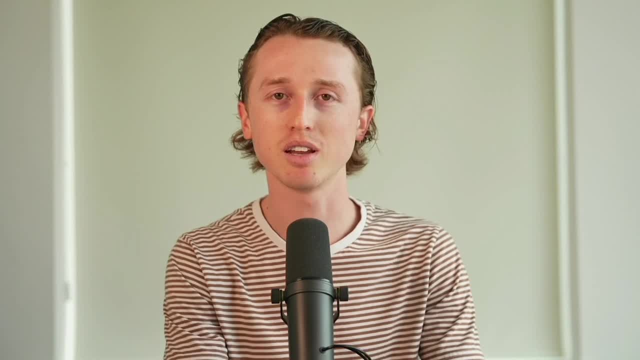 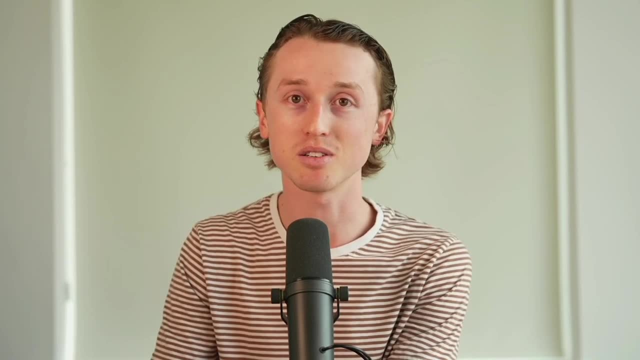 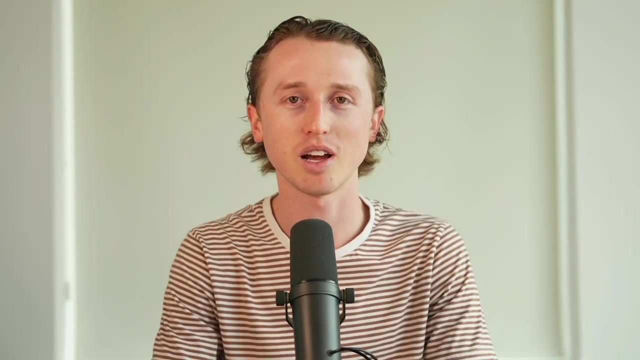 with it and replacing the time you would actually spend, you know, seeking god by thinking that you're you're healing and everything is going to come from stretching. but there are some people who need to stretch. there's some people who are in pain, some people who are have totally tight bodies and stretching helps them. i hope this video helped. 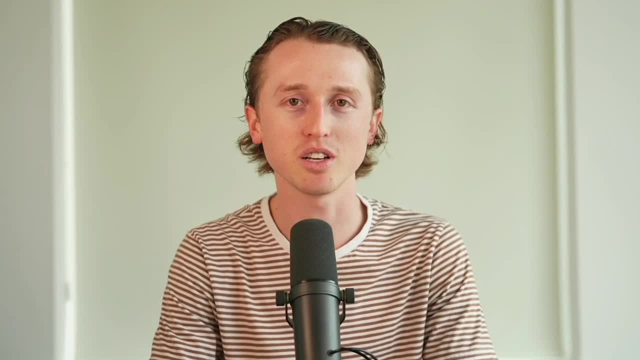 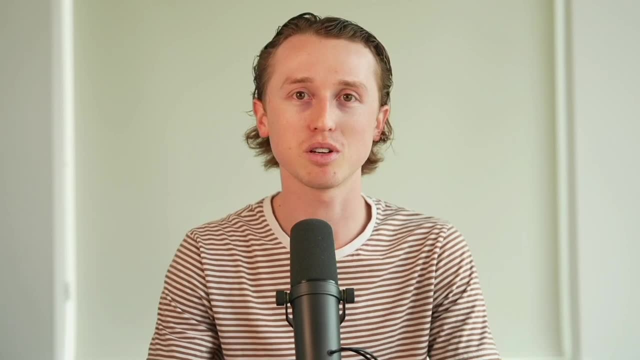 bring some clarity to this question, which is really a good question. you know you love the lord, you want to worship him. him only you shall serve, and not some hindu deities and hindu demons that you. you know we don't want to channel demons and you see, in hinduism they do this and this is 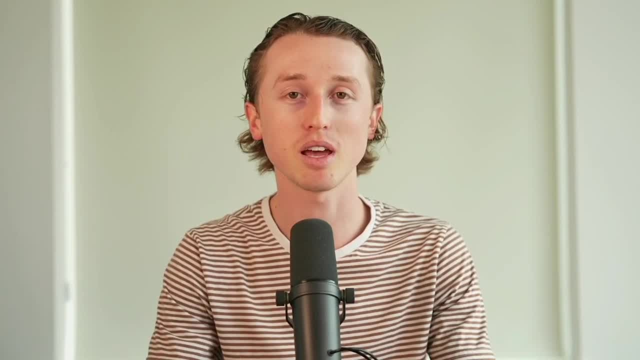 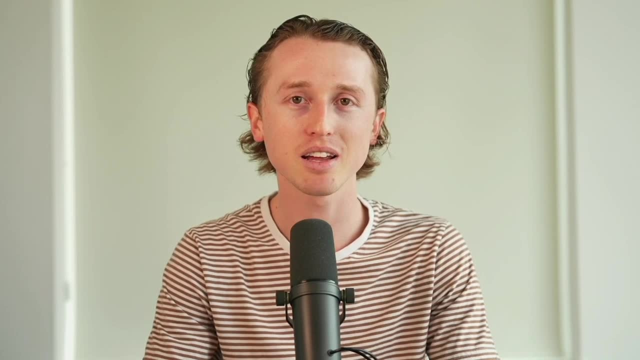 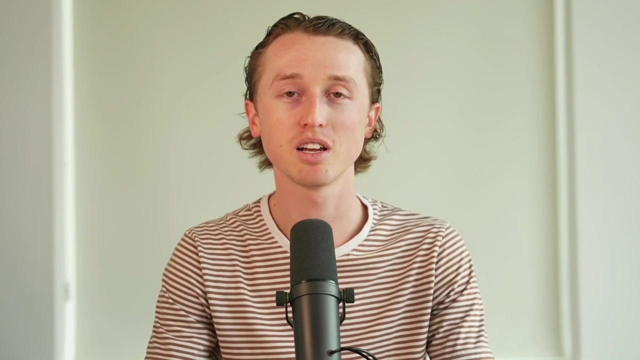 their beliefs and they want these spirits to inhabit them and help them and they worship these spirits. and you know you're like man but i like stretching like. is that bad? no, it's not bad and you could, even if you're bending down and touching your toes, but you're a satanist and you're telling a zazel, some demon, to come inhabit. 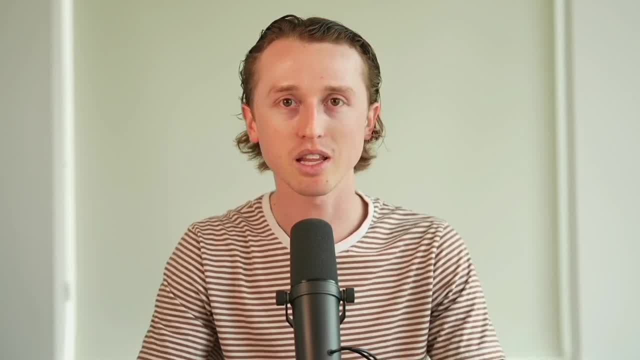 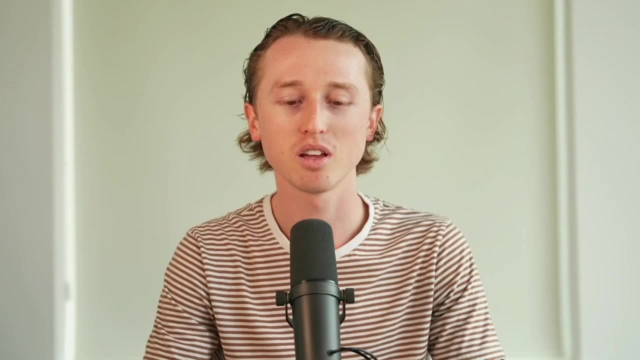 you right. when you touch your toes, you give it access. that's your beliefs, that's your, that's your pursuit. you go down, touch the toes and boom, you get. you get. you start channeling this entity, you get inhabited by this being. you could have that experience from touching your toes or you. 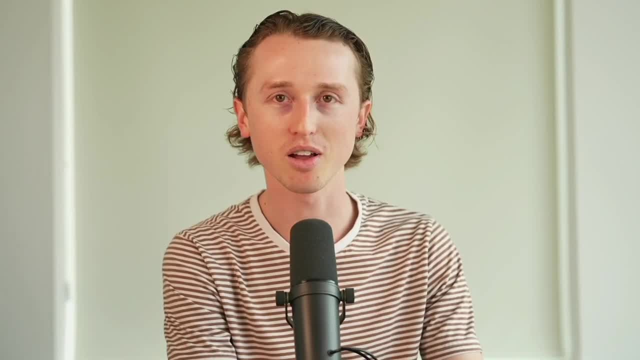 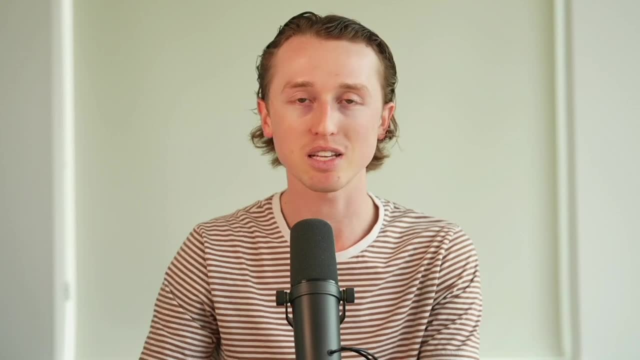 could just have the experience like before a football game: before you work out and you're stretching your hamstrings, nothing happens. it's the spiritual beliefs and the faith attached to them that matters. that's what matters in the spiritual realm in regards to a lot of these.